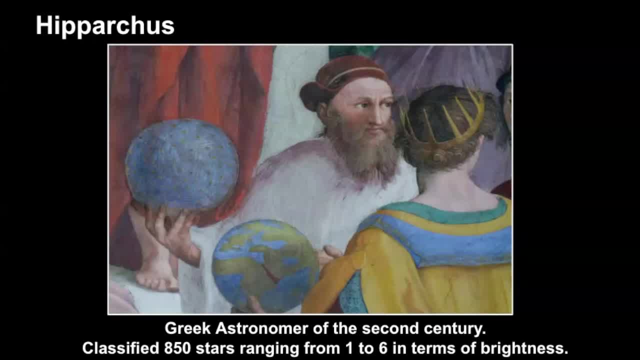 to be. From what we know at this time, Hipparchus was the Greek astronomer who lived in the second century, and he was the first to start this star brightness classification. He classified 850 stars, ranging from one to six in terms of brightness. So what did this look like for Hipparchus? If you 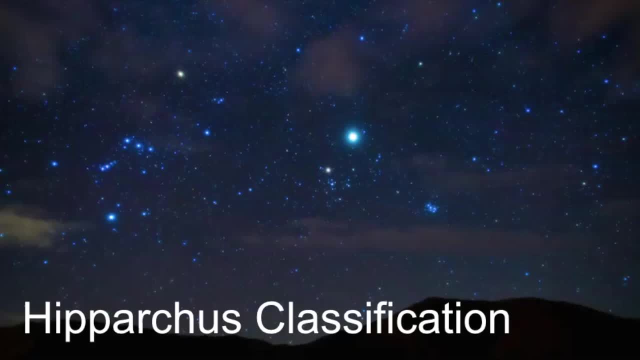 look at this picture here you can see that he was the first to start this star brightness classification. He said that there are a range of star brightnesses, So he said the brightest stars, like one Rigel, right here in the constellation of Orion, that would be a first magnitude star because it's very bright. 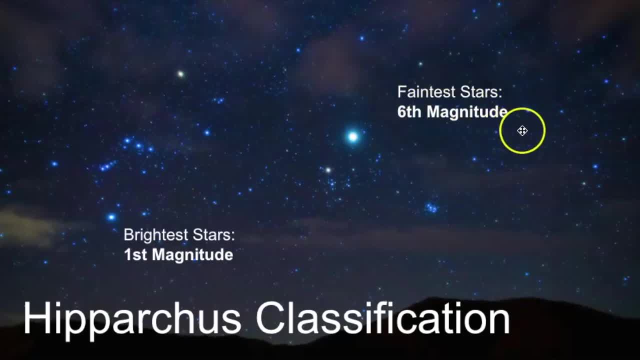 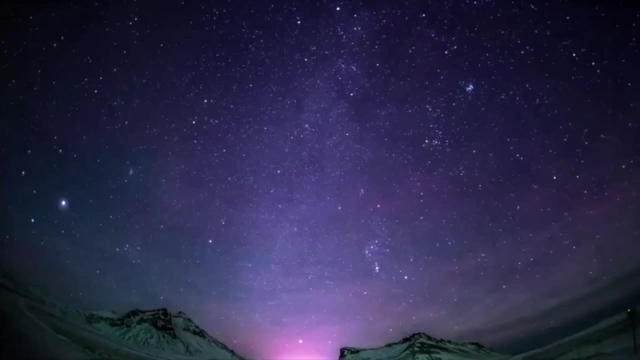 And then the fainter stars, ones that are up here that are very tiny little pinpoints and don't really stand out. those faint stars would be of six magnitude, And this was really used by Hipparchus. So as you look at this photo, you can see there are different brightnesses. And how do you? 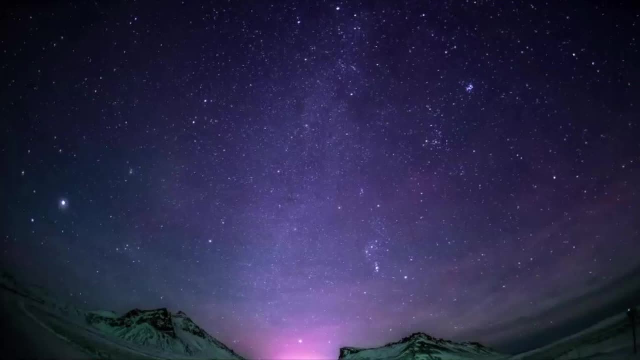 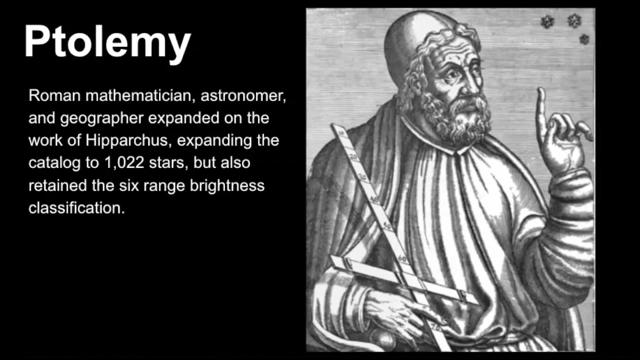 define them. There's a lot of questions here that I had, But what I did learn is that over time this system became a little bit more refined, also with the help of technology, of course. The next character we have in our story of star magnitude is Ptolemy, And he was a Roman mathematician and 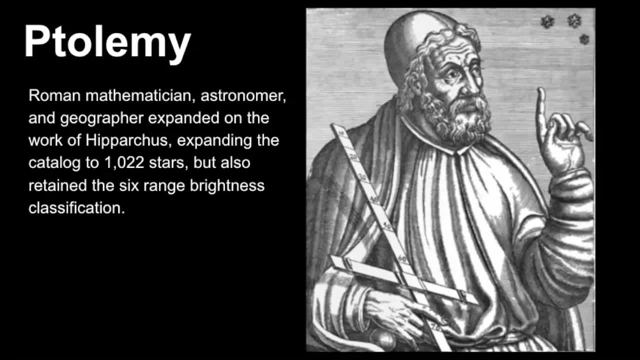 astronomer that expanded on the work of Hipparchus. He was the first to start this star brightness classification. He still retained that six range brightness classification, with one being the brightest and six being the faintest. But now we're going to fast forward towards Galileo's. 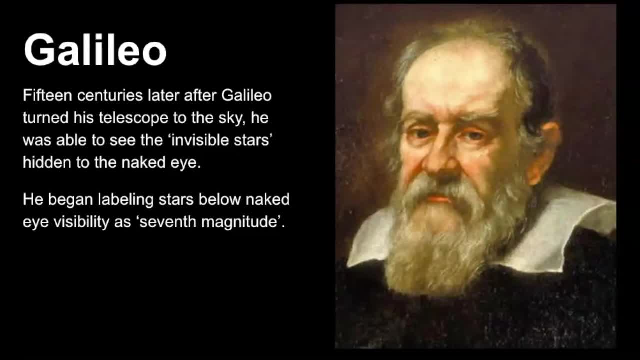 time, And when he looked at the night sky through his telescope, he was able to see these invisible stars, stars that you wouldn't normally see with the naked eye, because they're just too faint. So he started labeling these invisible stars as seventh magnitude. So he continued. 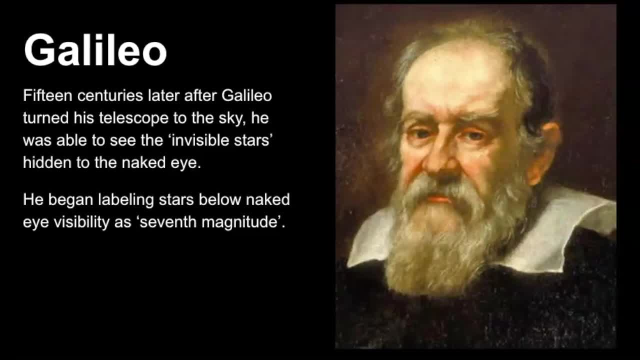 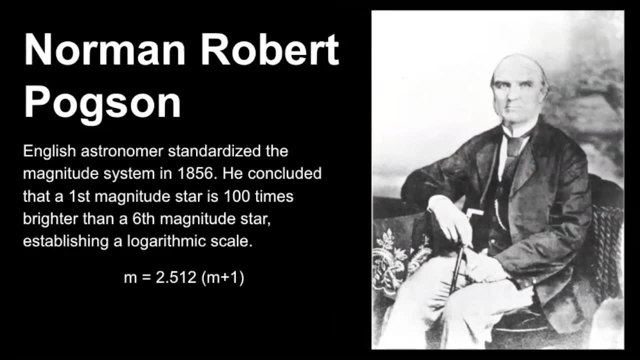 he continued Hipparchus' magnitude scale, but also expanded on it. Then we're going to skip on over to 1856. And an English astronomer known as Norman Robert Pogson standardized this magnitude system. because that's what scientists do: They standardize. we have to standardize our. 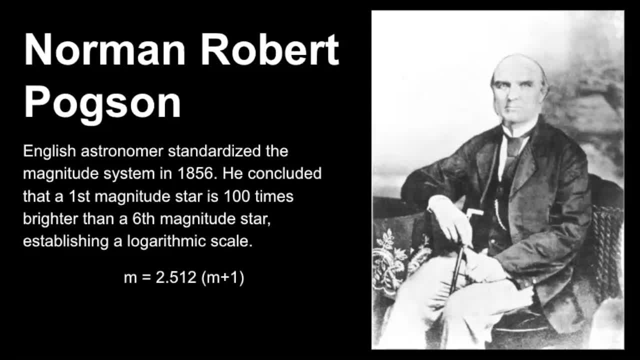 measurements, so we know what it is that we're measuring. So he concluded that first magnitude star is 100 times brighter than a sixth magnitude star and this established a logarithmic scale. But astronomers also look at magnitude from two different lenses and I want to explore that in the next part of this video. Another lens, that. 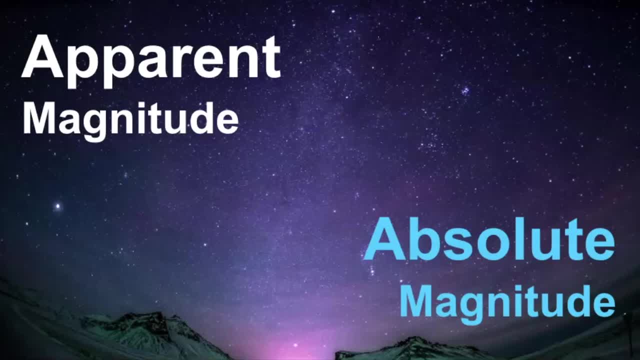 astronomers use in magnitude is the concept of apparent magnitude versus absolute magnitude. Apparent magnitude is probably what you're most familiar with, and that's the brightness of a star as it appears to us. But with absolute magnitude it's a little bit different. Astronomers will look. 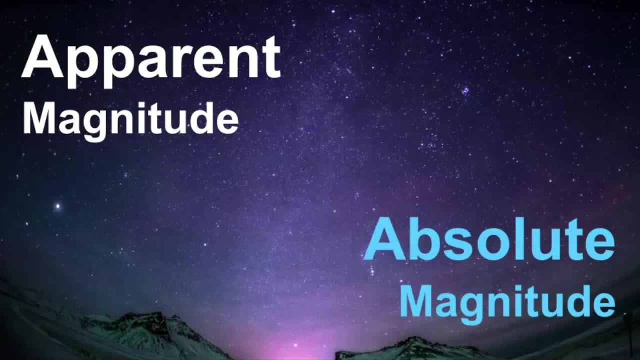 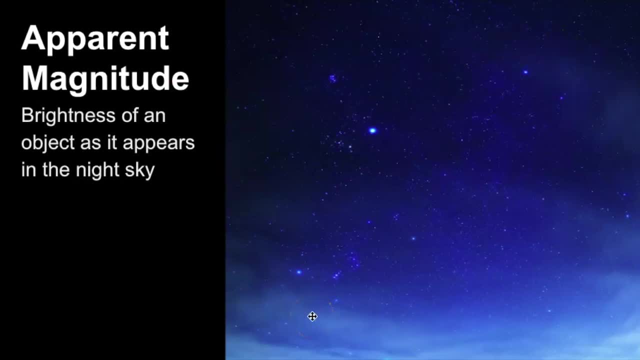 at the brightness of an object if it were at a particular distance. So apparent magnitude, as you're looking at this picture, is the brightness as it appears to us, the observer. So, for example, this is the Pleiades star cluster. That has a relatively lower magnitude, which means 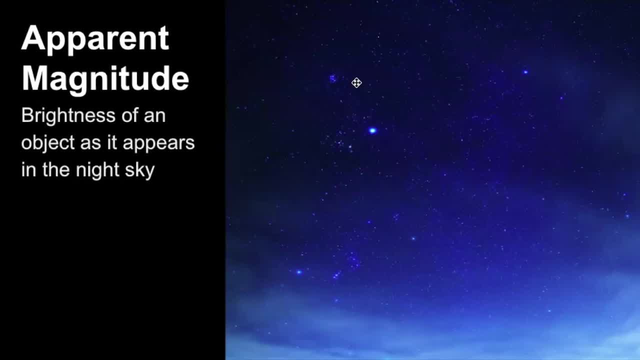 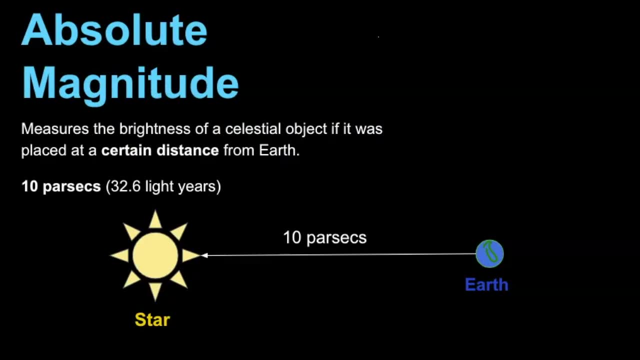 it's brighter, and we're going to explore this scale in a little bit, so stick with me. But absolute magnitude is when scientists will measure the brightness of a celestial object if it was at a particular distance from Earth, that distance being 10 parsecs. So if we're here on 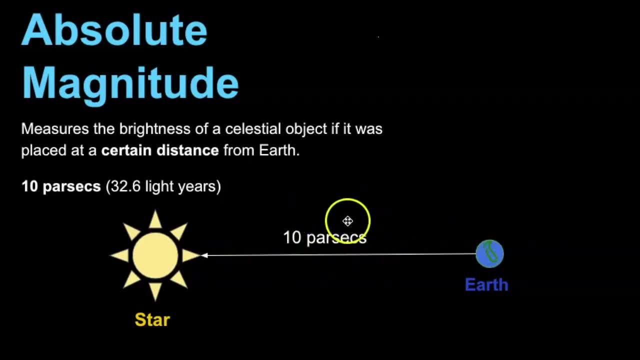 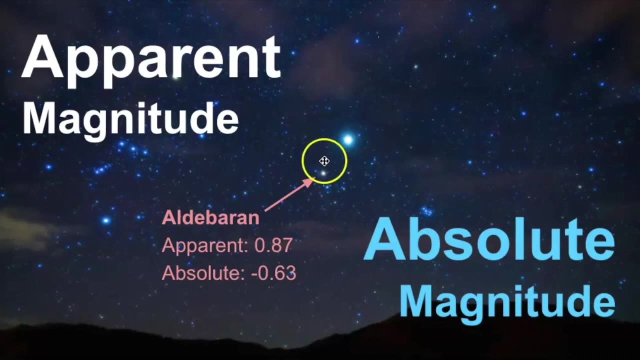 Earth and a star was placed at 10 parsecs away, 32.6 light years- how bright would it be? So we can have two different values for magnitude based upon the lens at which you're looking at. So let's get an example of this. So this star right here, this is Aldebaran in the constellation of Taurus. 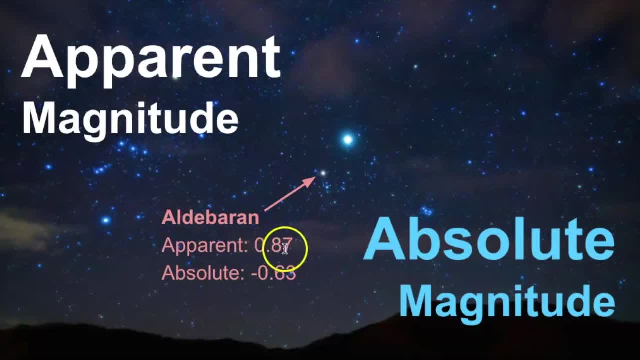 it has an apparent magnitude of 0.87.. So very close to one which tells us it's a bright object but its absolute magnitude is negative 0.63.. So this seems confusing because it's like: oh, does that mean it's brighter or dimmer? So I do want to go ahead and explore the difference. 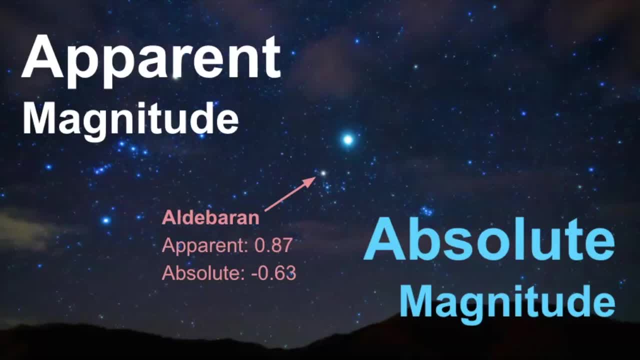 between the negative, Which are usually brighter numbers, and then the positive: the bigger the number, the dimmer it is. But I wanted to just go over this concept of Aldebaran having two different types of magnitude, one being what we see from our perspective and one being if this star was placed at a particular 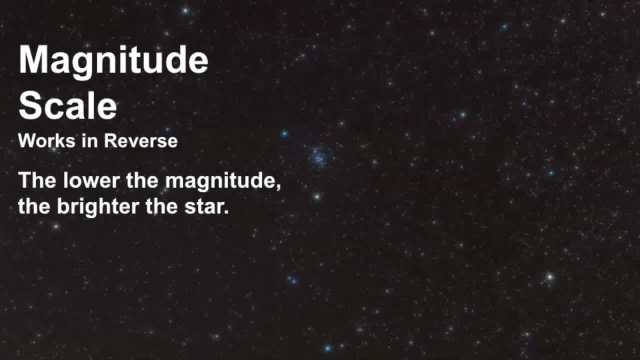 distance, what would the brightness be? So let's take a look at some of the examples of different stars we see in the sky versus what their magnitude would be- And I'm purely speaking of apparent magnitude. Remember, the scale works in reverse, So the lower the magnitude, the brighter. 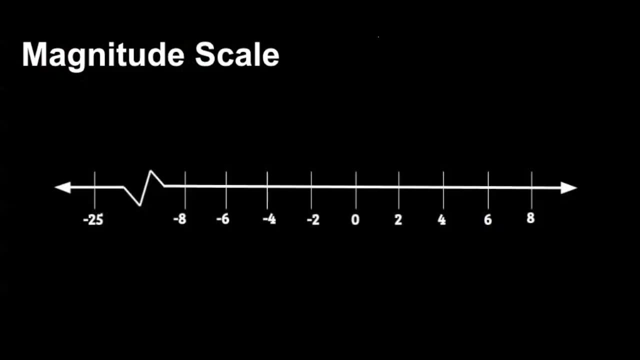 the star. So let's take this timeline, or number line, I should say, and we're going to place some different stars on here and show you where they lie. So first we'll start with Vega. Vega is in the constellation Lyra. I have a video about that. go check it out, And it has a magnitude of zero. 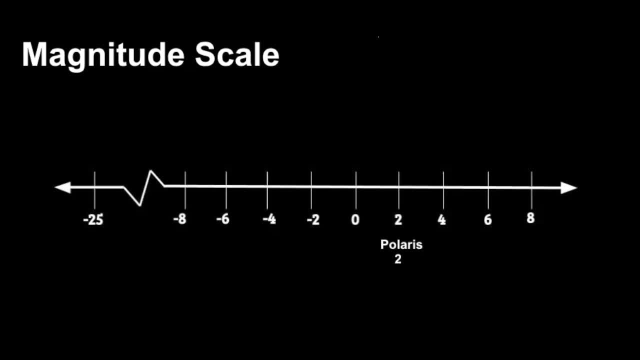 which tells us it's a pretty bright object in the sky. But if we look at a star like Polaris, Polaris is the North Star, the star that doesn't appear to move. I've got a video on that, one that has a magnitude of two. So Vega is brighter than Polaris, even though the number is bigger. 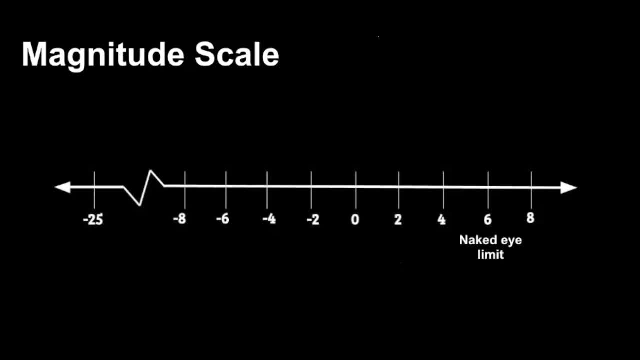 with Polaris. Remember inverse relationship. Our limit that we can see with the naked eye is six. So anything at a magnitude six is the limit that we can see. If you start going to seven, eight, nine, you need magnification to see anything. 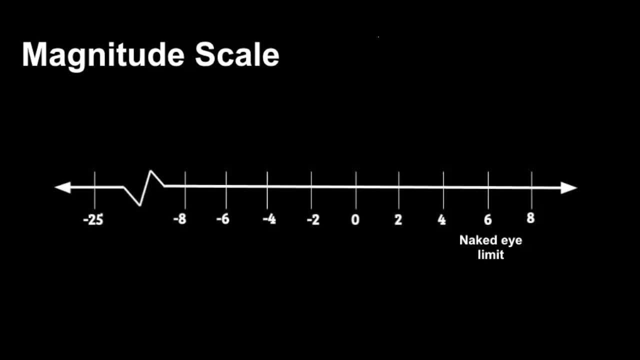 That is above a six If we keep going here. Sirius: the brightest star in the night sky in the constellation Canis Major. I've got a video on it. go see it if you want to learn more. That star is negative 1.5. So it's really bright. when you compare it to say, well, I don't want to say 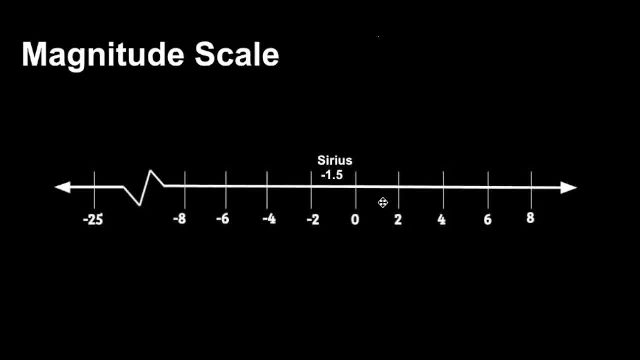 really, really bright, And I'm not going to get into the mathematics of this, But if we bounce back to Polaris, Sirius would definitely be brighter than Polaris. If we keep going, Venus, a planet now that we're speaking of, has a. 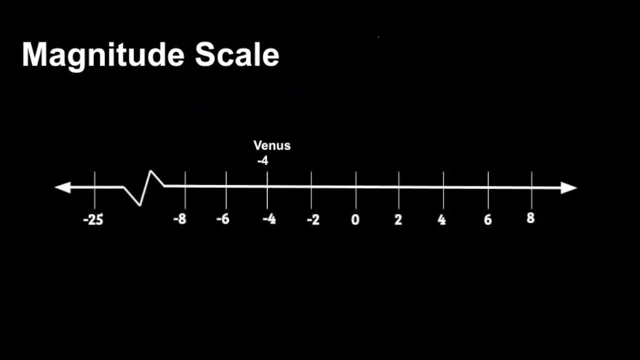 magnitude of negative four. So that tells us Venus is really bright in the sky. I can always tell where Venus is because it is the brightest object in the sky next to the sun, which the sun has a magnitude of negative 27.. So that seems counterintuitive, right? 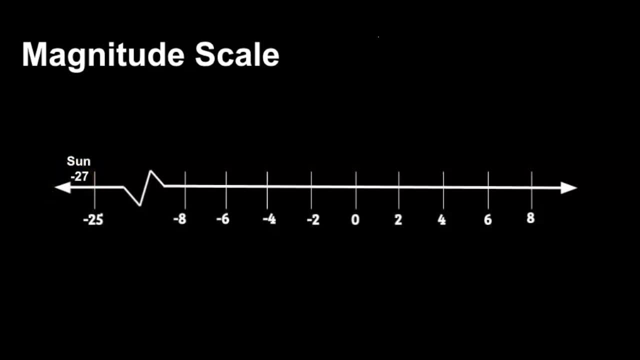 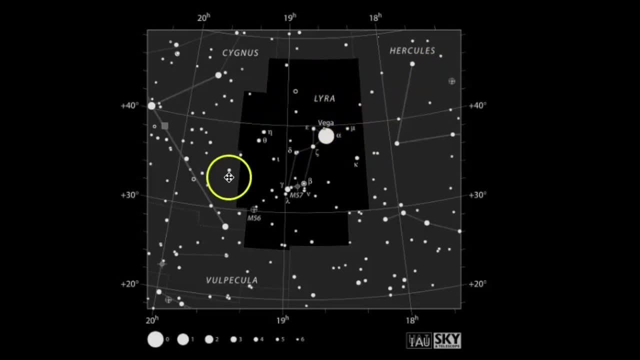 That negative means it would wouldn't be as bright. But remember, Venus is the brightest star in the night sky in the constellation Canis Major. So if we take a look at a star map here we're going back to Vega. Vega is the brightest star in the constellation of Lyra. 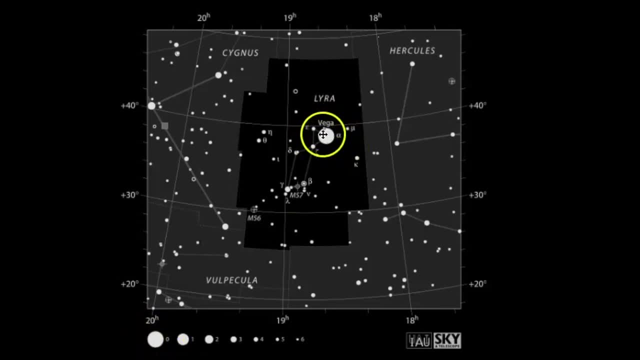 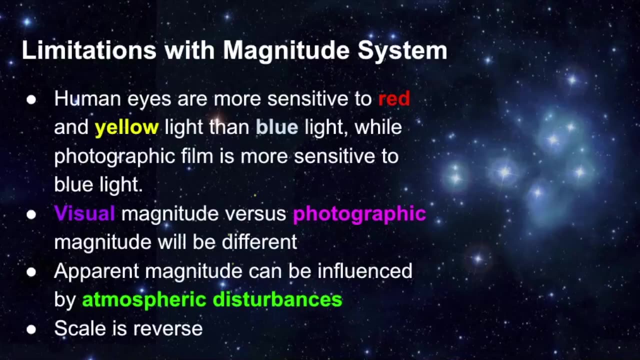 And you can see the magnitude scale down here. We defined that Vega was zero magnitude and you can see its size matches that magnitude. So that's how it works. Okay, we know there are some limitations of this, So some of the limitations include human eyes. 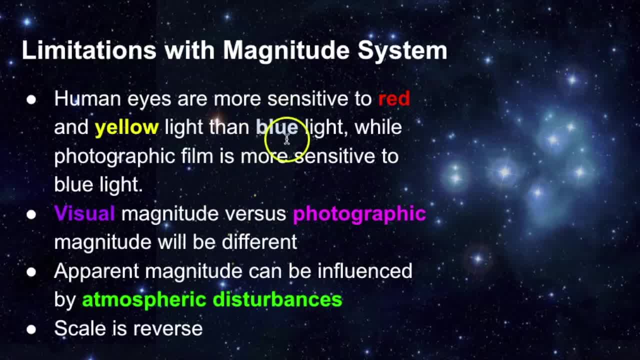 We can see that the eyes are more sensitive to color and yellow light than blue light. As you can see, I did color this blue, but it doesn't stand out as much as red and yellow And also photographic film is tends to be more sensitive to blue light, as you can see in this example. 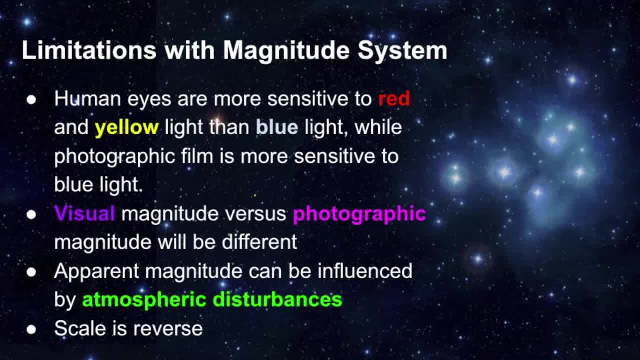 So another limitation is that visual magnitude versus photographic magnitude will definitely be different. We are limited by our human eyes and we can capture things on photographs that we wouldn't be able to see otherwise. apparent magnitude that can also be influenced by atmospheric disturbances, So you can see this if 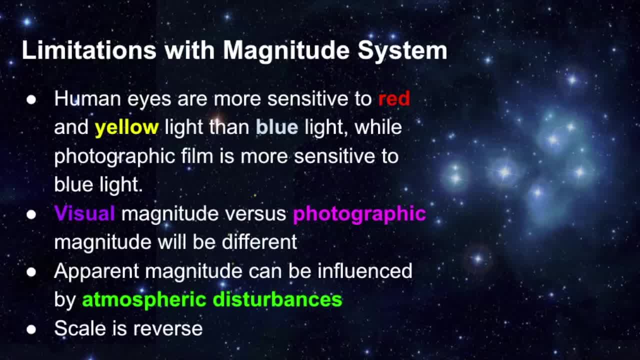 you look at stars that are right up along the horizon, what you see is this kind of twinkling going on, And that's really the gases moving in the air that causes that twinkling, And it's usually more pronounced along the horizon And also the scale is in reverse, So that can make 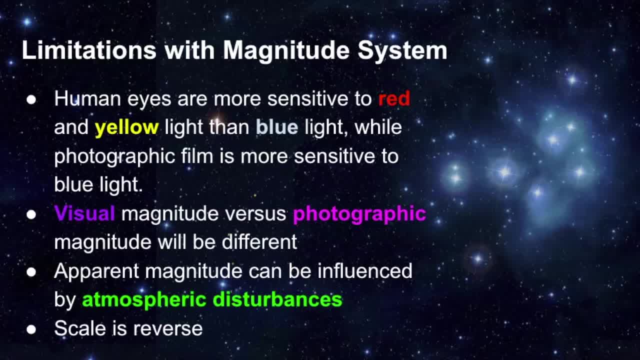 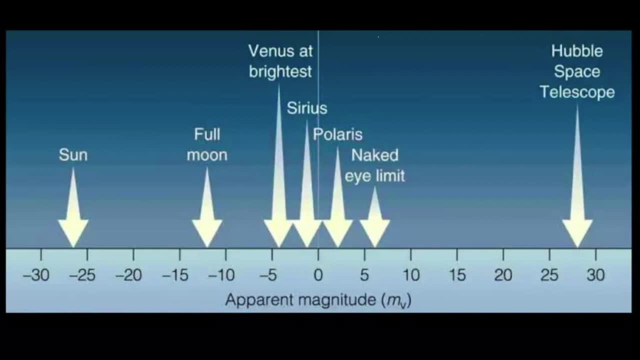 it confusing as well. So if we wanted to see what's what is like the absolute greatest- or I shouldn't say absolute, that might be the wrong choice of words, But how far can we see out there with the instruments we do have today? So I found this picture and I find it interesting because it 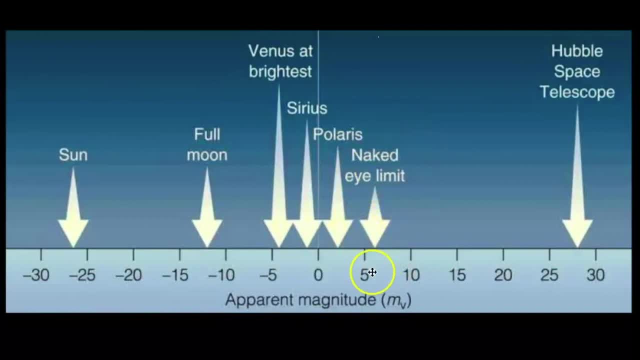 shows you the naked eye limit, which is magnitude of six. notice we're talking of apparent magnitude. the Hubble Space Telescope sees a little more than 25, in between 25 and 25.. And it's a little bit more than 25.. And it's a little bit more than 25.. And it's a little.